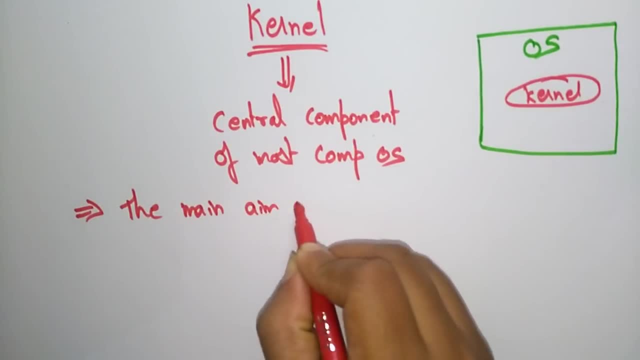 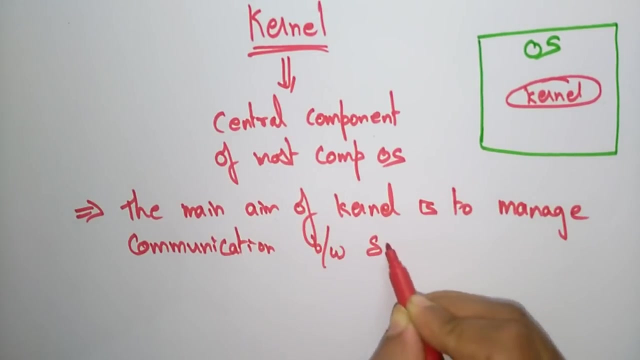 The main aim of kernel is to manage communication between software and hardware. So this is the main aim of kernel. It is just just like an operating system. Actually, the operating system is aim is also to manage the communication between the hardware and the application program. Okay, so this is the main aim of kernel. 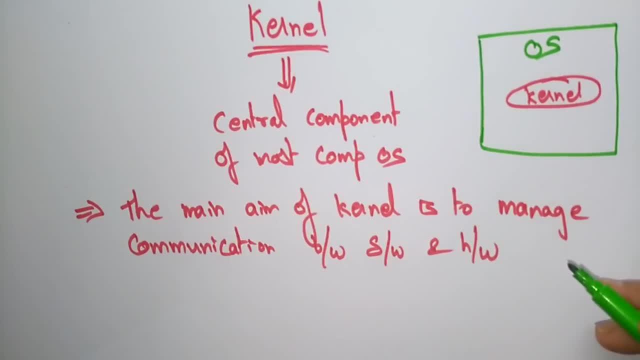 But kernel is a part of the operating system which is responsible for translating the commands. So whatever the commands that the hardware and the software has to be done. Okay, so this is the main aim of kernel: to manage the communication between the software. A software is nothing but the user level applications. Let us take it is a user level applications, The, all the user level applications, or comes under the software, whereas the hardware is nothing but the CPU. 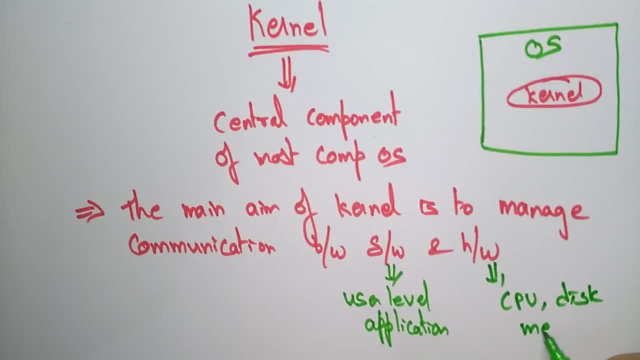 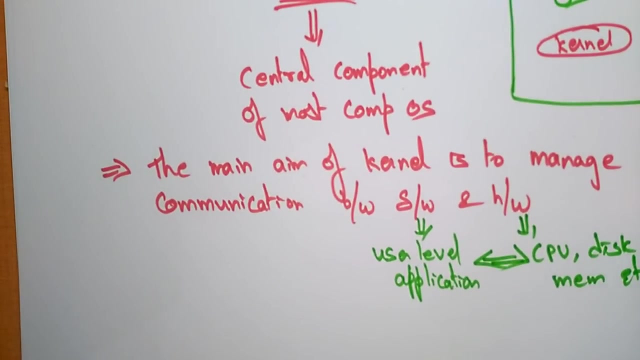 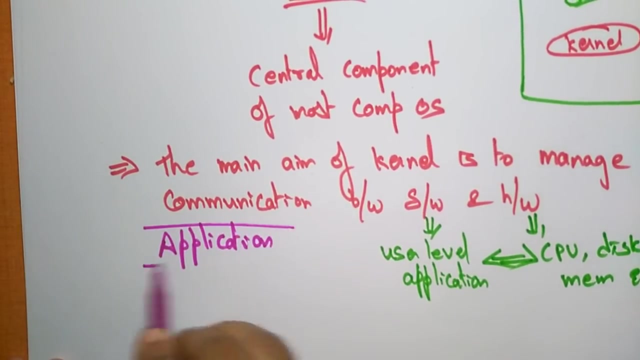 This, or even the memory, etc. So this is a hardware. So the aim of kernel is to manage the communication between the hardware as well as the software. Let me show you clearly. Let's take: this is a user level applications Application. Okay, so this is a user level application. Let's take the hardware. That is a software. 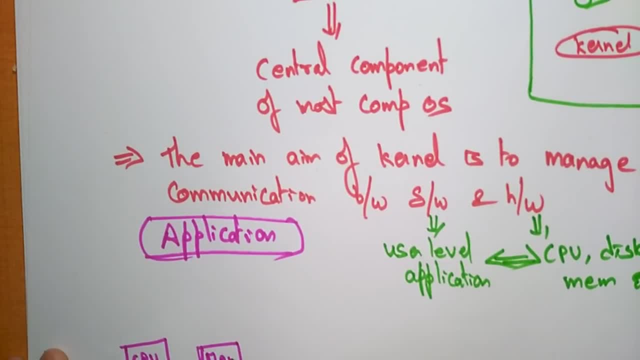 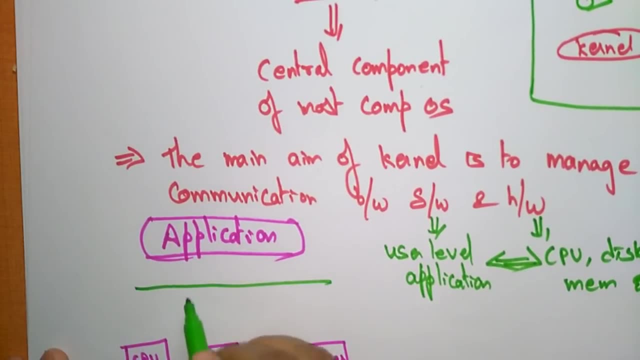 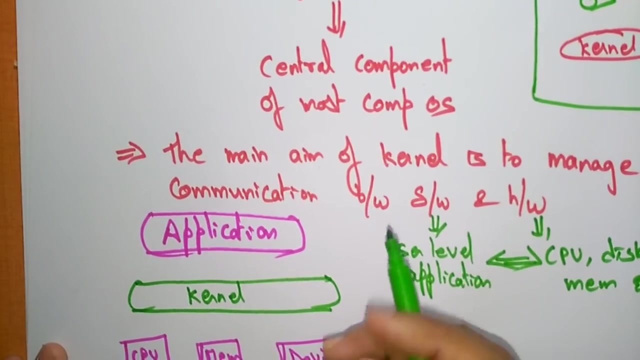 The CPU memory and even you can take the devicesrio devices. So in between that you are having the kernel. So this is nothing, but it's an operating system. So just a part of the operating system. So access and interface between the user level application as well as the hardware. So that's a part of the operating system. 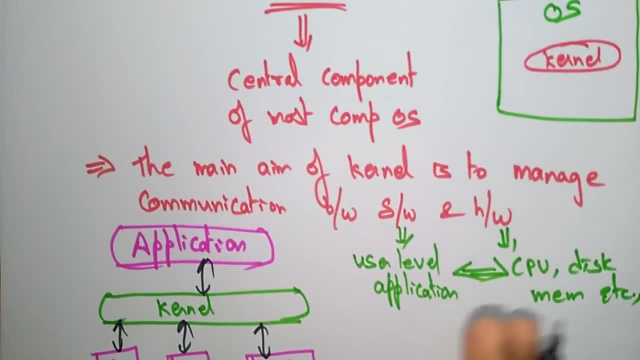 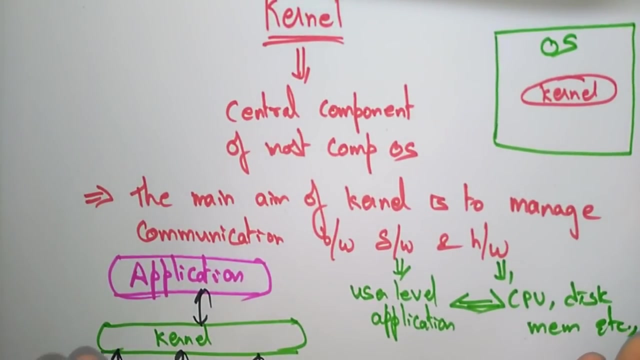 is a kernel. so whenever you asked about what is a kernel, you just tell a kernel is a main part of operating system which is responsible for translating the commands that can be understood by the computer. okay, so this is the definition of kernel. okay, so what? uh, how this is related to our 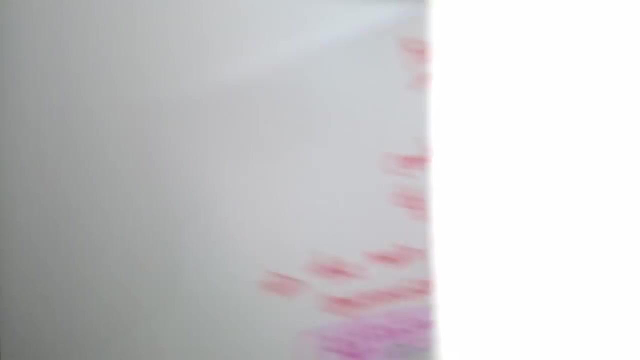 embedded system, okay. so, uh, whatever the embedded systems you are taking, that every embedded system is acting in the real time. okay, so, wherever you are using that embedded system concept, so that should be a real-time application. so now let's see the real-time kernel. let's take 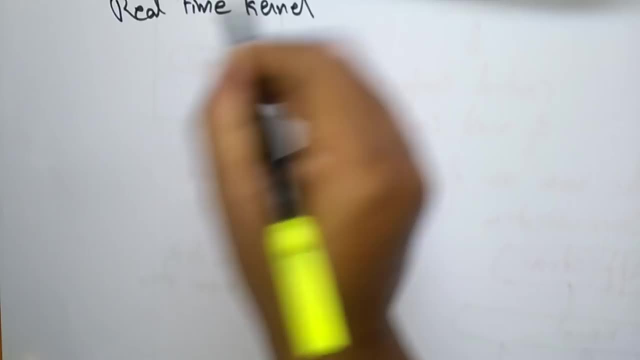 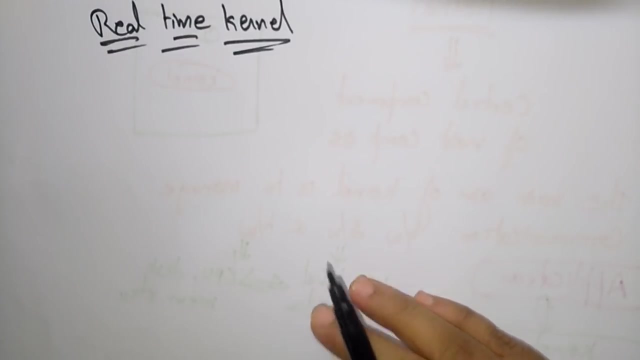 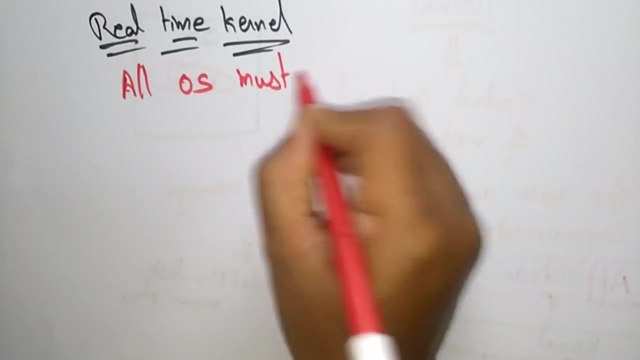 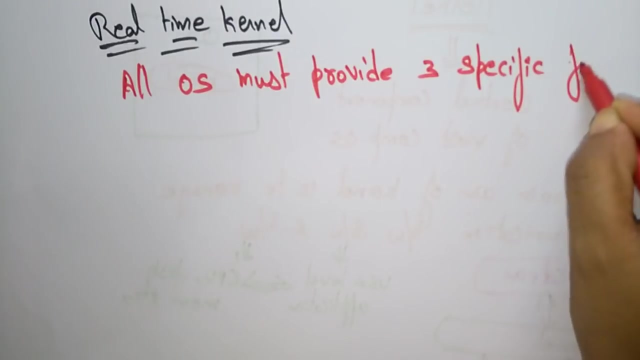 the real-time kernel. so i hope you understand the definition of the kernel. so then, what about the real-time kernel? actually, all operating system must provide three specific functions. so, whatever the operating system we are taking, okay, so that operating system, all operating system, must provide three specific functions. so what are the three specific functions? 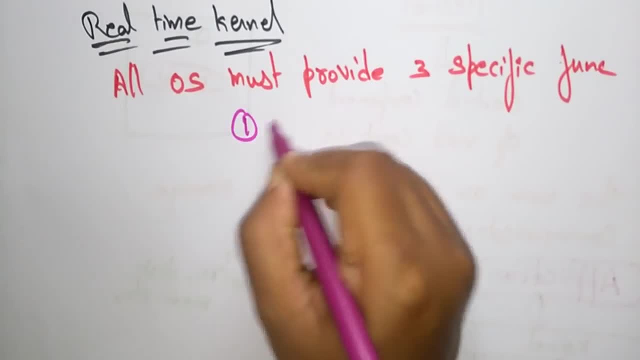 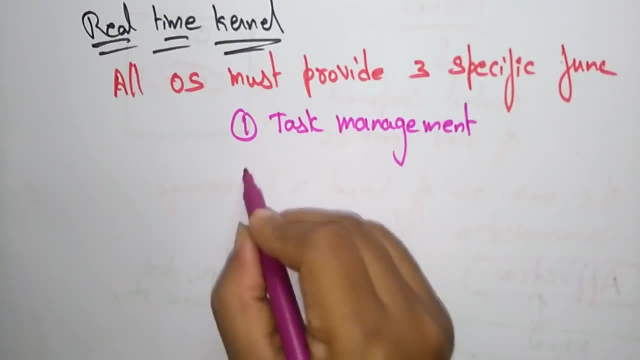 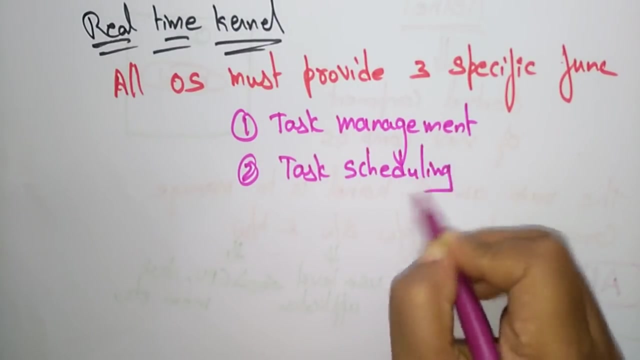 that the operating system must provide. one is task management- task management. second one is task scheduling and inter-task communication, inter task communication. so these are the three main functions that any operating system should provide. so all these task okay, so is also done means it's just: uh, a kernel is the smallest portion of the operating system. 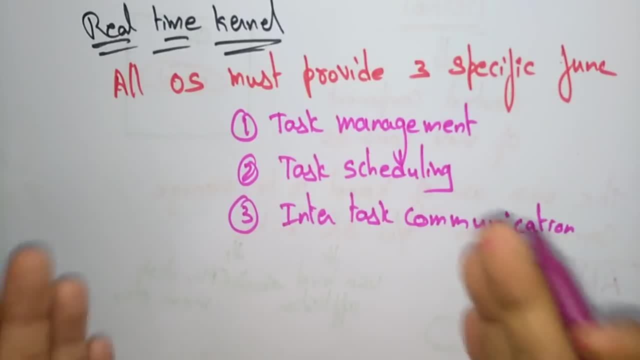 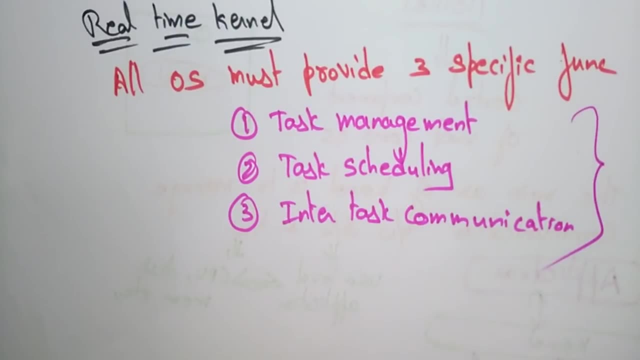 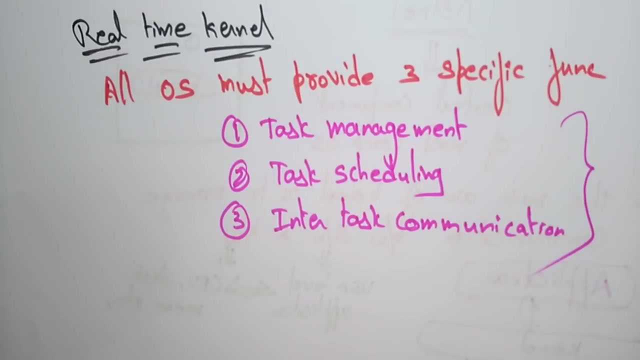 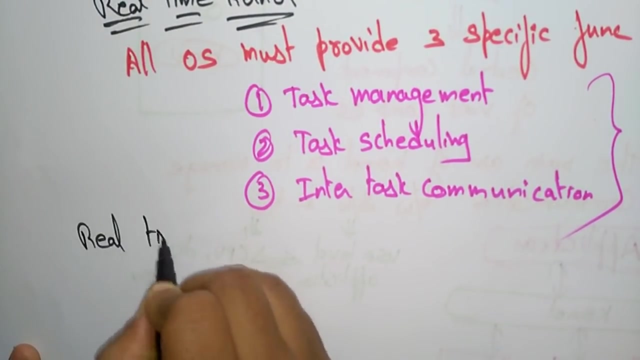 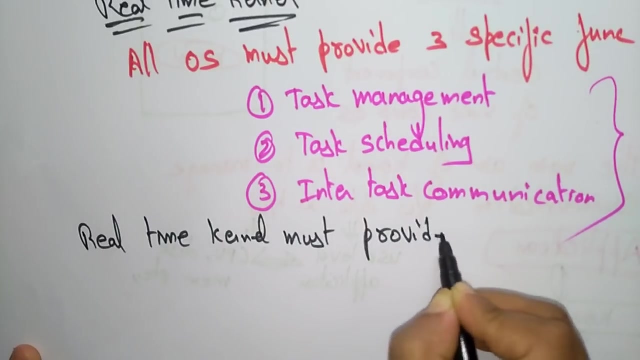 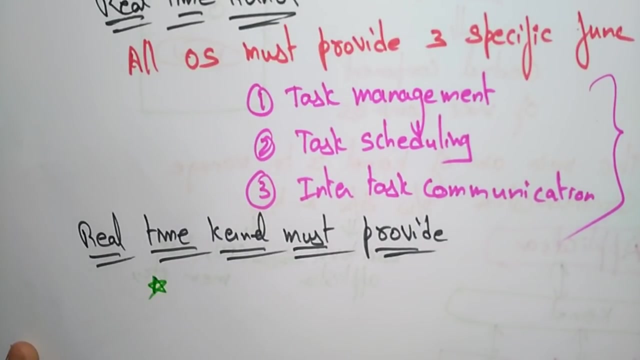 So it's just a kernel is the smallest portion of operating system. We know that That provides all these functions. The kernel is going to provide a task management, task scheduling and inter-task communication. So real-time kernel must provide Real-time kernel must provide one interrupt handling. It is going to provide interrupt handling. 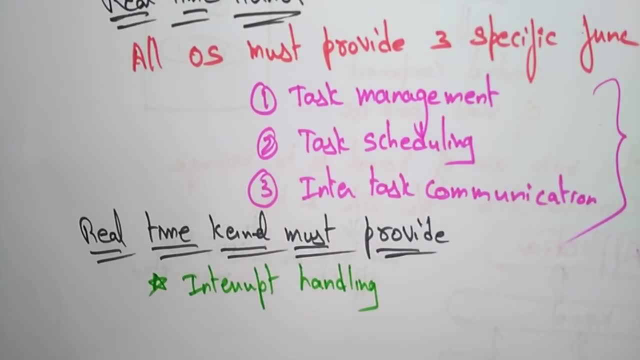 So these are all the features of the real-time kernel. So what exactly that real-time kernel is providing along with these? So the kernel is going to perform the task management, task scheduling and inter-task communication, So along this thing. So it is going to provide a features like interrupt handling, So guaranteed interrupt response will be there, and process management.